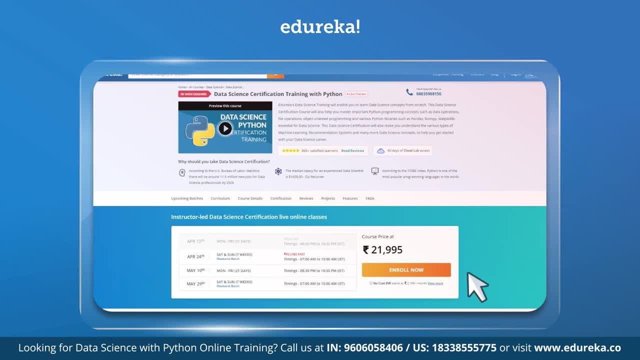 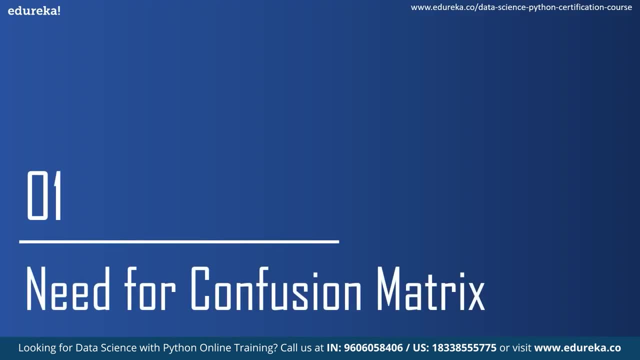 and hit the bell icon to never miss an update. Also, if you are interested in online training, certification, do check out the link given in the description. Alright, so now let's start For understanding what is a confusion matrix. we will take a step forward and understand. 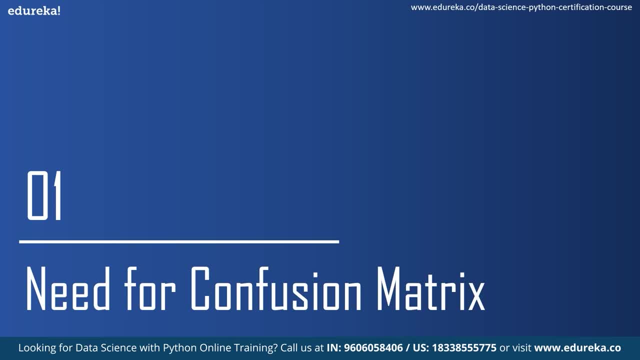 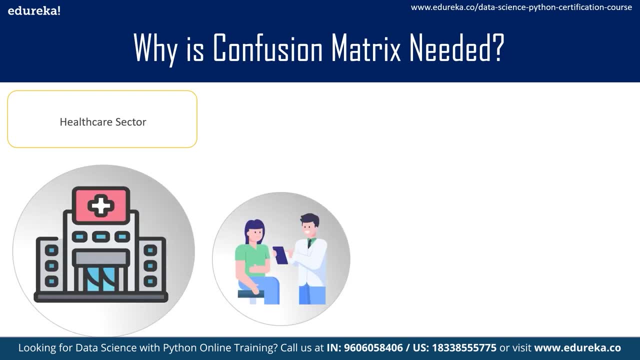 the need for a confusion matrix. So let us understand this with a short story. We will take a healthcare sector and suppose a patient visits a hospital and the doctor examines the patient and says that the report is all fine and the patient is healthy and just prescribes. 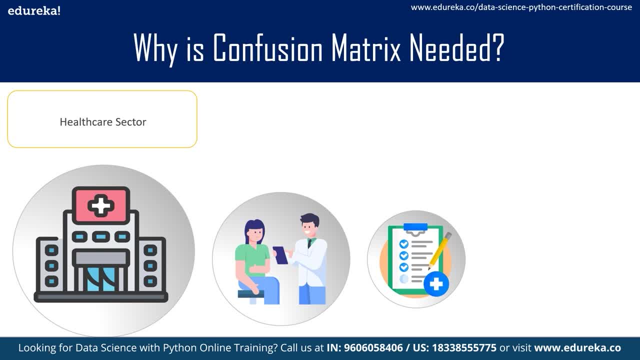 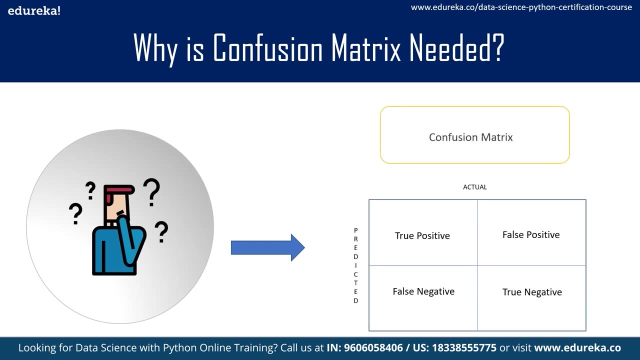 a few basic medicines, But what happens is that after a few months, this patient is admitted to the hospital with severe conditions and is fighting for life. What went wrong here? Well, you must be guessing what is confusion matrix has to do with all these things, So 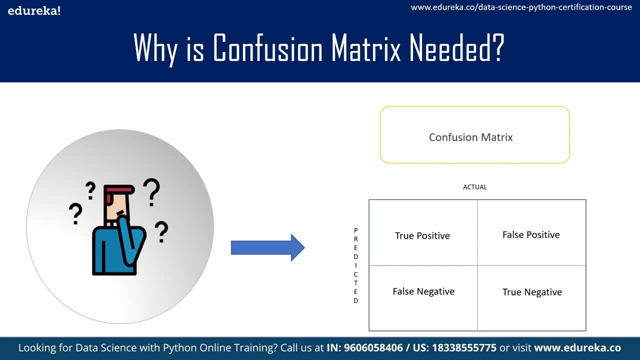 confusion matrix here helps to figure out the misclassified cases. that means here the doctor missed out the patient who is having a heart disease. So confusion matrix really helps us to not to miss these crucial cases, especially in the healthcare sector. this is really very important. So now let's understand it a little better. why do we need it? So now, 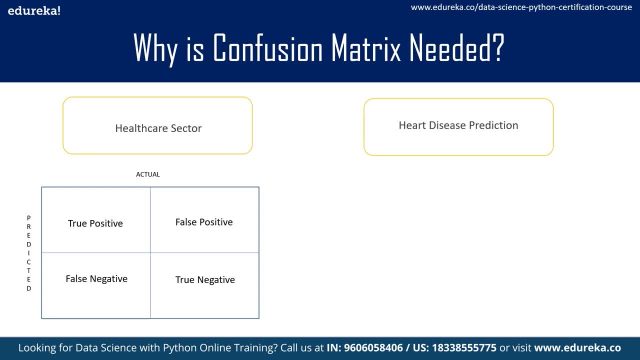 let's suppose In the healthcare sector we have this confusion matrix and we have to predict a health disease, prediction whether a person has a heart disease or not, and the classifier is the doctor or the algorithm. we will change interchangeably classifier or algorithm and we will treat. 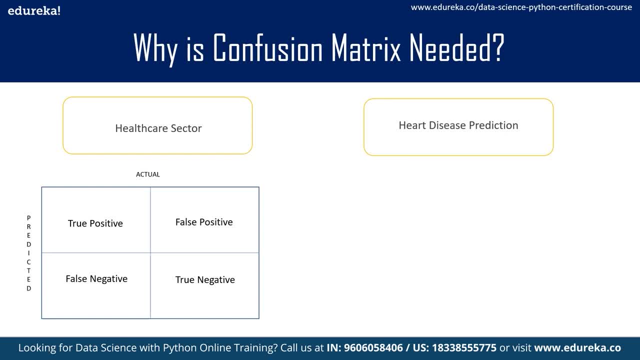 it as doctor. So now what happens is that the doctor predicts whether the patient is having a heart disease or not, and which means that if it is a wrong prediction then we have got errors. So let's just get a basic understanding of these things. 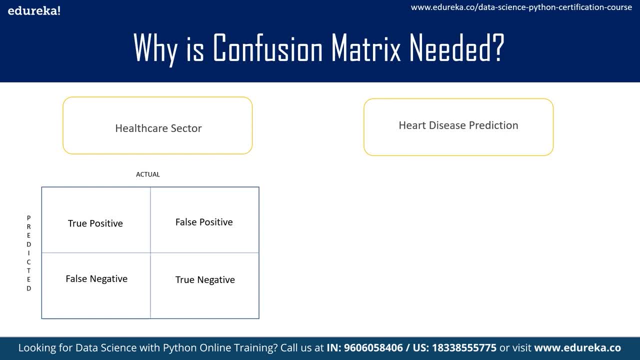 So now what happens is that the doctor predicts whether the patient is having a heart disease or not. So let's just get a basic understanding of these things and we will understand them in depth. but this is the crux of confusion, matrix. So let's understand this false, negative. 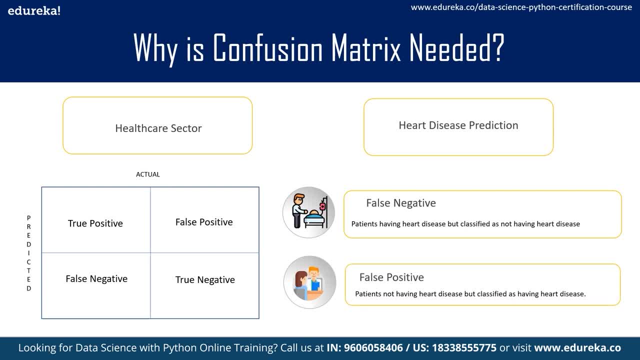 and false positive cases. Of course, the true positive and the true negative cases are the cases which are rightly predicted by the doctor. That means a person who is having a heart disease is true positive and person who is not having a heart disease is true negative. 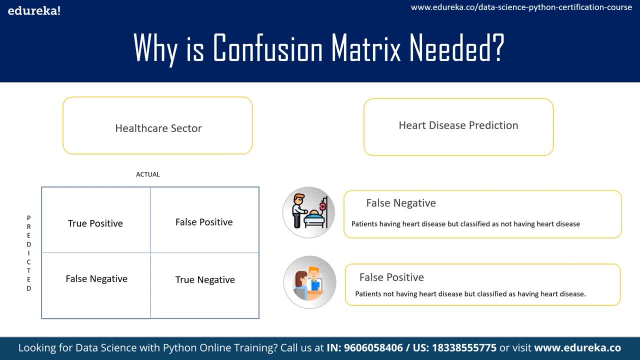 So the doctor classifies them correctly. But what happens if a doctor classifies a patient wrongly- So the patients who are having heart disease, but they are classified as not having a heart disease? it is called as false negative, as we have seen in this case, and this was. 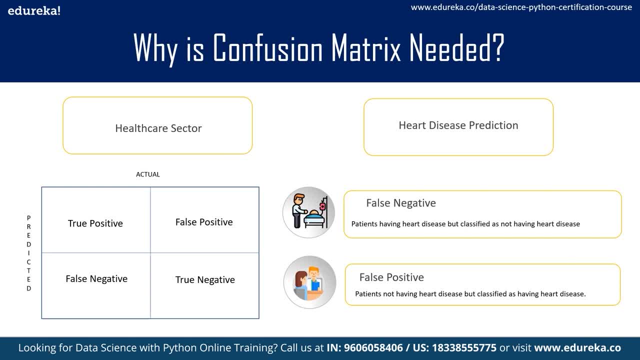 a question of life and death for the patient. On the other hand, the false positive cases are the patients who are not having heart disease, but they are classified as having heart disease. So confusion matrix give us an estimate of all these cases and we can really check whether the algorithm is performing good or not. It is a kind of a report card. 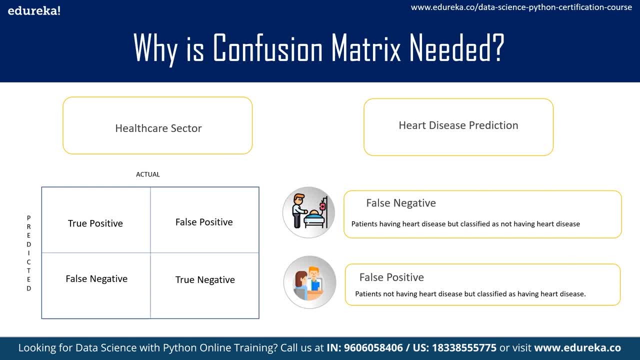 for the algorithm So we can check the correct cases and the misclassified cases. So that's why we need a confusion matrix, to get a complete evaluation, the overall report of a classifier. So now, having said this, we will break down this concept bit by bit and understand confusion. 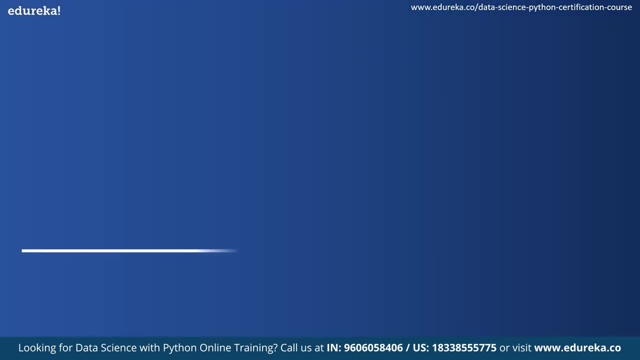 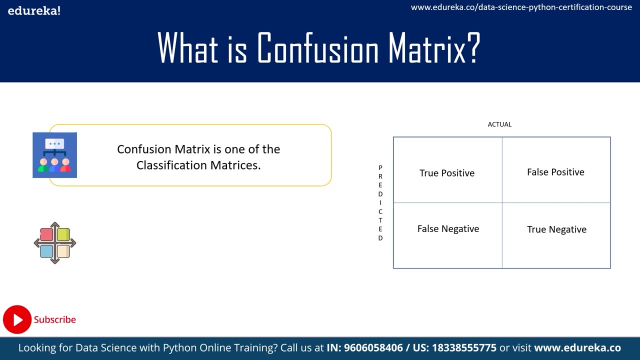 matrix from scratch. So now moving on forward to understanding what is a confusion matrix. So confusion matrix is one of the classification matrices apart from log loss, accuracy or area under curves. These are the other classification matrices, but today we will study about confusion matrix, and confusion matrix is used for evaluating the performance of 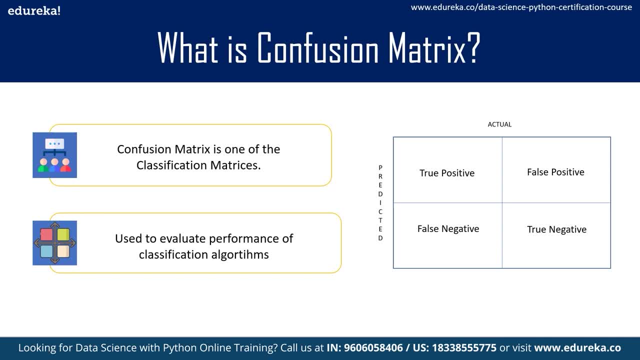 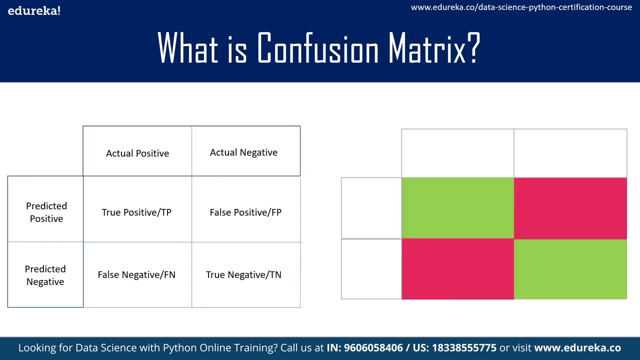 classification algorithms. So now, classification algorithms are like navbase, svm, knn or logistic regression, even random forest for that matter. So how these algorithms are performing can be evaluated with the help of confusion matrix. So now let's understand the confusion matrix. 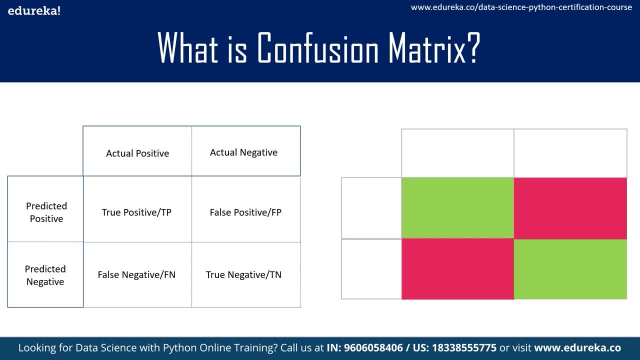 So what we see here is two confusion matrix, but on the right hand side we see some green and red boxes. So the green boxes indicate the right predictions made by the algorithm and the red boxes indicate the errors or misclassified cases by the algorithm. So now what happens here is that this will no longer be confusing once we will. 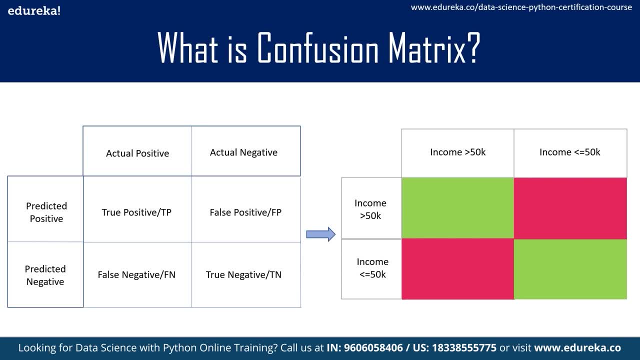 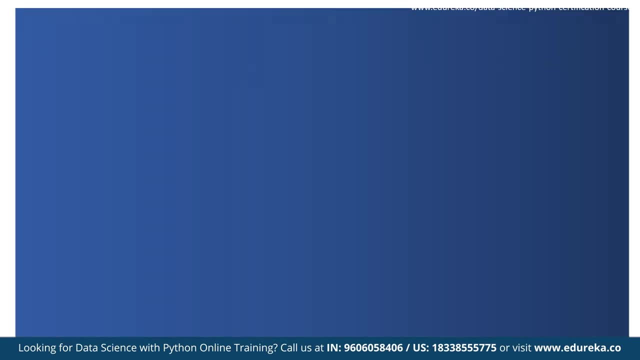 understand this with the help of this example, wherein we have to classify people into two groups: having income greater than 50,000 and less than 50,000, or less than equal to 50,000.. So let's now take our understanding to our next level, to understand this with the help of an example. 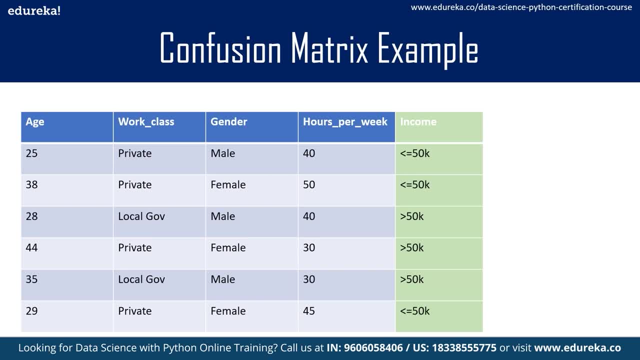 So now we will proceed on with this example. This is again a small subset of the data taken from the census data and this is having five features, like five columns and six rows. So here we have got features like age, which is having different age groups and work class, like 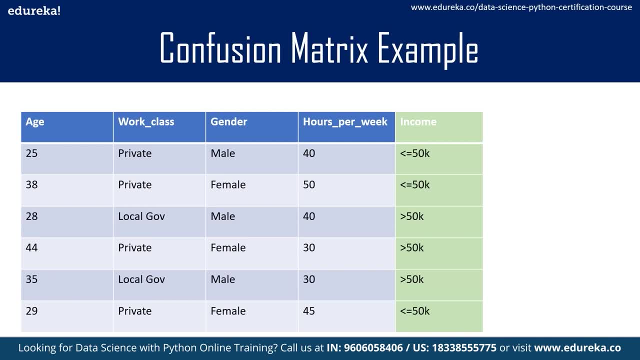 private and local government. We've got gender- two genders are here, male and female- and hours per week. it is 40, 50 depending on the hours per week- and based on all these things, we've got a target or the output variable, that is, income, which is less than. 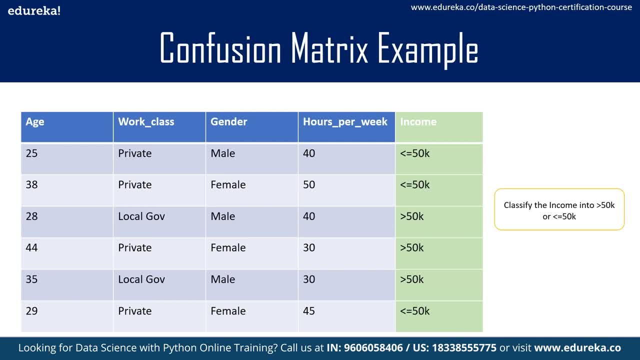 equal to 50,000 and greater than equal to 50,000, and our task is to classify the income into these two respective groups. Now, this is completely a binary classification problem and, since we've already got an output here with our data set, this is a supervised machine learning problem. 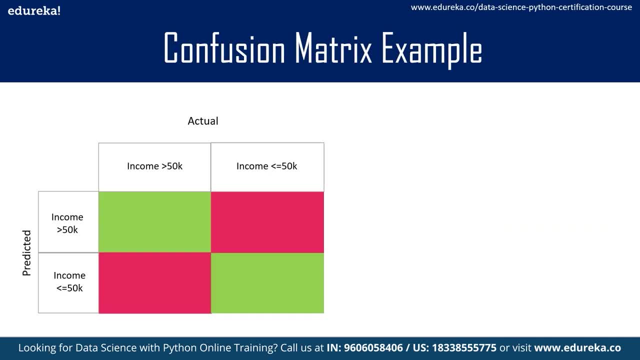 Alright, so now let's move on to confusion matrix. So here we see a two by two confusion matrix, and again this is for a binary classification problem. Of course the confusion matrix size would increase, given the multi-class classification it could move on to even further. you know it's not. 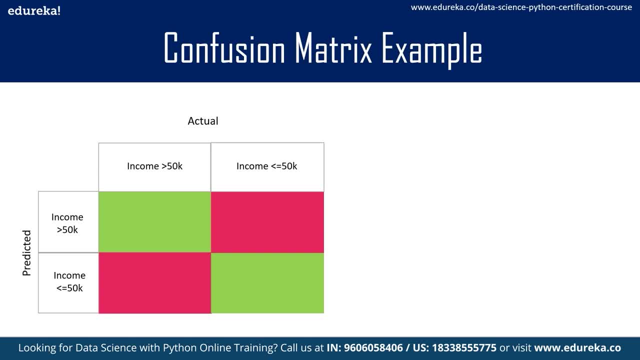 necessary that it will be two by two. it could be n into n also. So now this confusion matrix, let's understand the basic one now so that we can take it on further to a higher level. So now, what happens here is that the actual values we see, actual values, the columns in confusion matrix are the 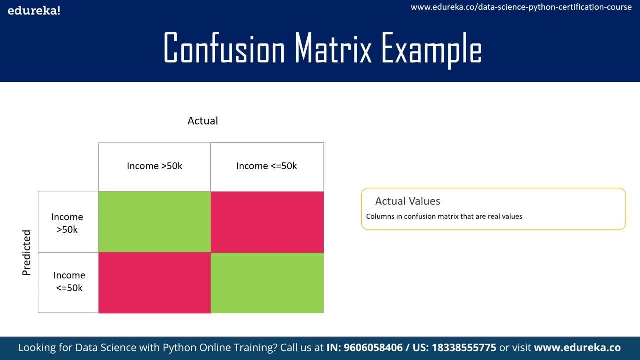 actual values. that means these are the real truth values in the data set and these are true values That our data set has. and these are the predicted values which are depicted in the rows. that means these values are being predicted by the algorithm and when the actual and the predicted values 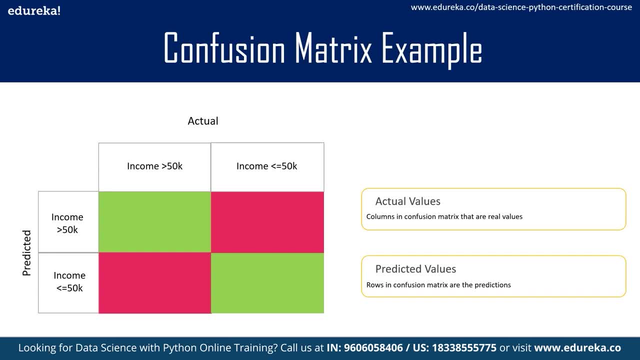 they match, then it is a correct prediction, and when they do not match, it is an incorrect prediction. So we see here that when the actual and the predicted values match, it is being showcased by the green boxes, and when they do not match, it is being shown by the 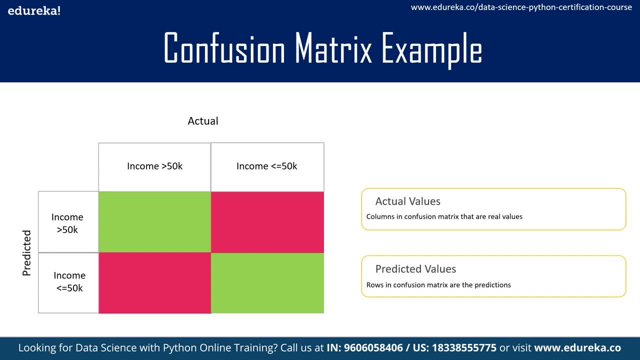 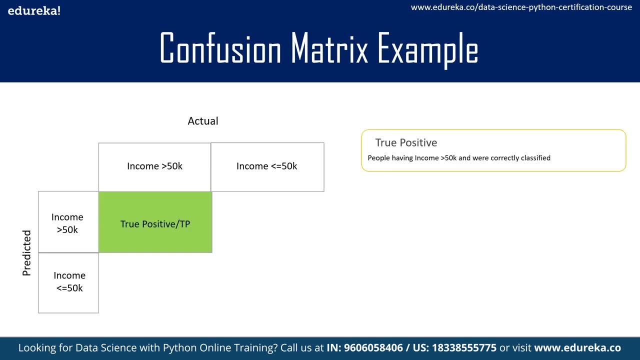 red boxes, right. so now let us understand this by again, by filling it up. okay, so now we see true positive. okay, so now i'm filling the cells. so what is this true positive? true positive is nothing, but it is just actual value when it matches the predicted value. so for here, in this example, 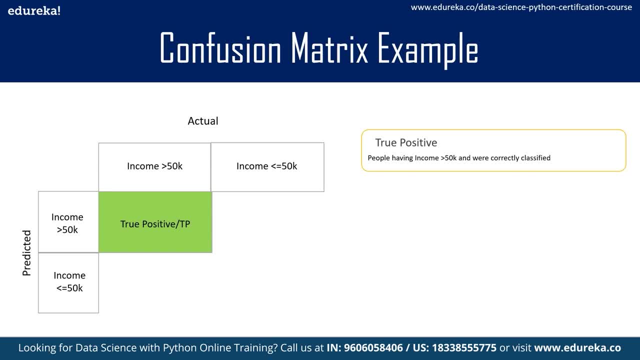 the people who were having income greater than fifty thousand. they were correctly classified by the algorithm as under the group having income greater than fifty thousand, so that becomes true. moving on forward, for another correct prediction was true. negative. that means people who were not having income greater than fifty thousand. that means i can say that people were having income. 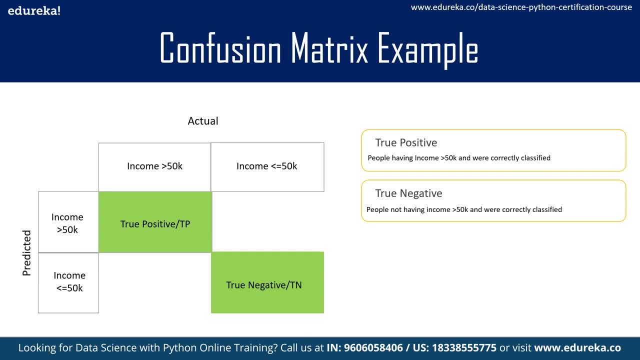 less than equal to fifty thousand. they were correctly classified into the another group, which was having income less than equal to fifty thousand. okay, now we move on to another. now this is a misclassified case by an algorithm. this is false, negative, which means that people who were having income actually greater than 50 000, but algorithm predicted it as less than equal to. 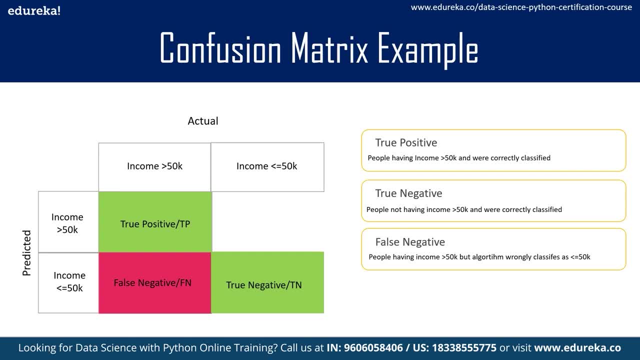 50 000 and this error- false negative- is also known as type 2 error. now, moving on forward to the false positive, and this is known as type 1 error. here the people who were not having income greater than 50 000, but they were predicted as or classified as income group having greater than 50 000. so the 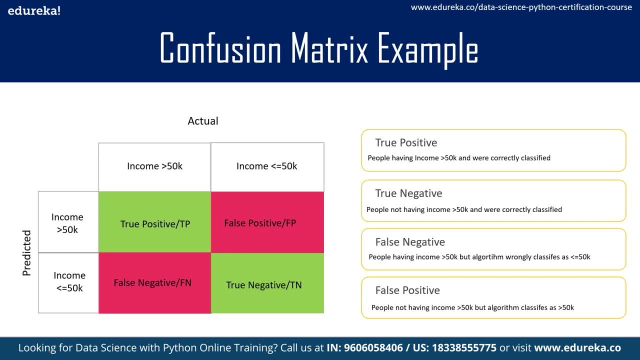 actual income group of these people were less than equal to 50 000, but our algorithm classified it as greater than 50 000. so these are the real meaning of true positive, true negative, false positive and false negative. whereas false positive, we have already said that it is a type 1 error and false. 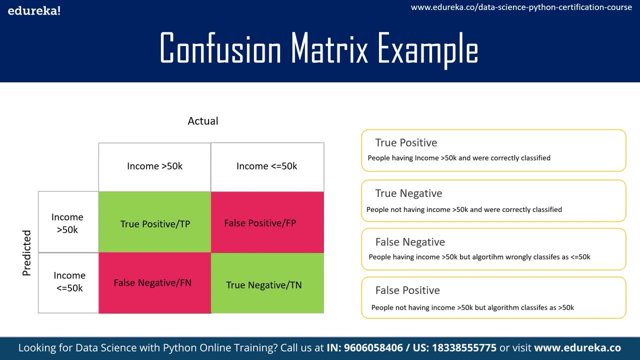 negative is the type 2 error made by the algorithm. all right now. so confusion matrix shows us the correct and the incorrect predictions, and this also helps us to evaluate the performance of an algorithm. so let's see how it does it. so these are certain values which have been filled and we 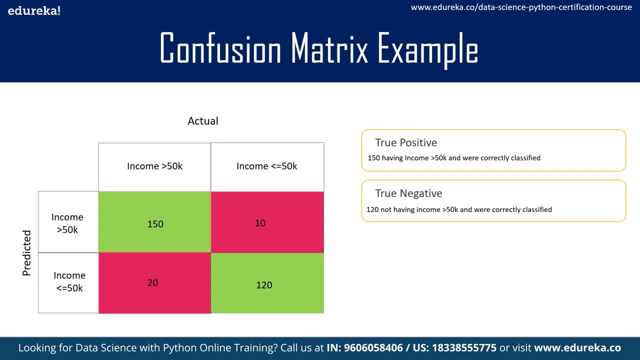 know that the true positive and true negative here. so let's calculate true positive. so here we see that 150 cases are correctly classified by the algorithm into the correct group of income having greater than 50 000. right and true negative are the cases for the people having income less than. 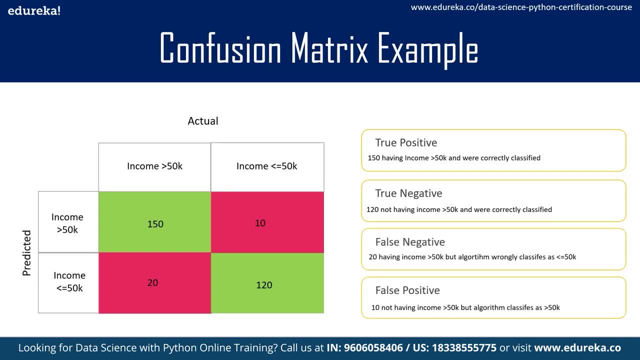 equal to 50 000. so now coming to false negative, so there are 20 people who have been misclassified as people having income greater than 50 000, but the algorithm classified it as income having less than 50 000.. similarly, it applies to false positive also, wherein 10 people were not having income. 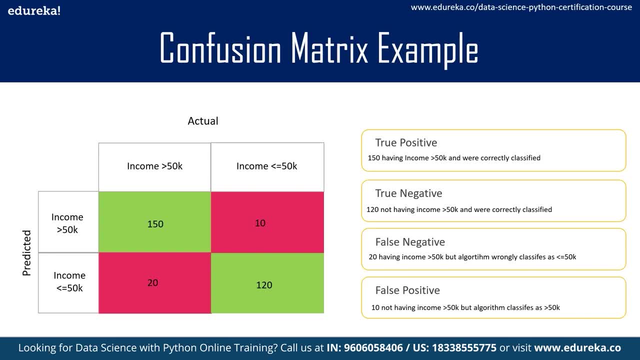 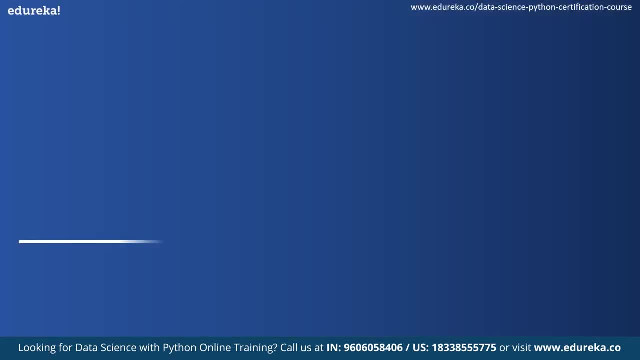 greater than 50 000, but algorithm classified it as greater than 50 000.. so these are the misclassified cases and this is how we fill it now, moving on forward to understanding few matrices in confusion matrix. now let's see how we fill it now moving on forward to understanding few matrices in confusion matrix. 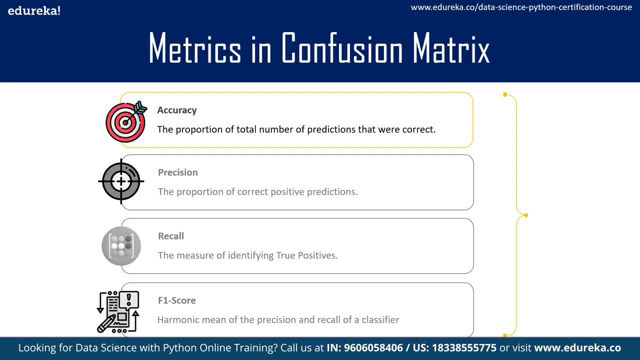 here. the first one is accuracy. accuracy is nothing but the proportion of total number of predictions that will correct. so let's take an example of accuracy and understand it with the help of an example. so here we see again the same confusion matrix and we will calculate the accuracy from. 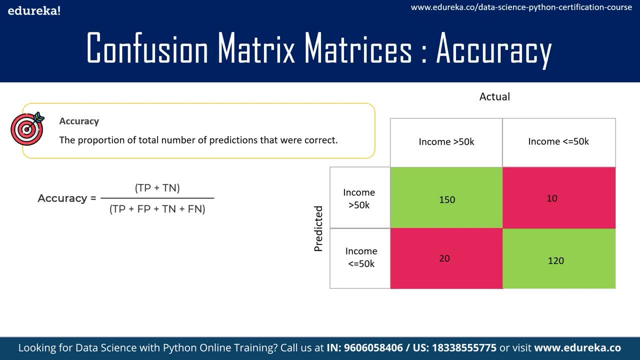 this matrix. so the formula is true positive plus true negative divided by the total number of predictions by the algorithm. so now we see here that accuracy comes out to be, after filling the values, that is 90 percent. so now we see here that accuracy comes out to be, after filling the values, that is, 90 percent. 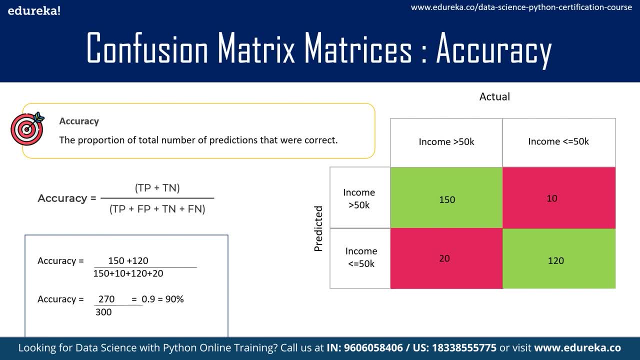 so now, one thing to note for accuracy is that this is one of the matrices in confusion matrix which we are deriving out from confusion matrix. it is not explicit, but it is implicit, and by filling in the values we get accuracy. and this is accuracy, is actually not suitable. 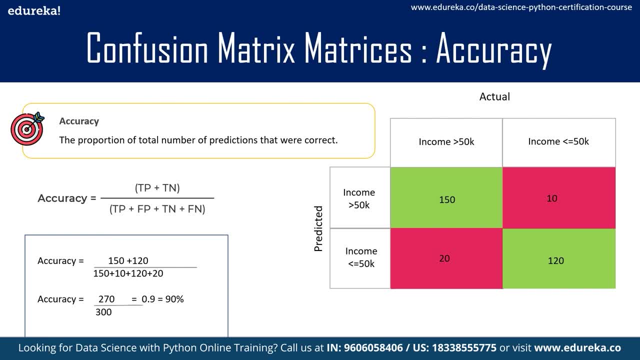 for imbalance data sets. it is suitable for balanced data sets and it gives the measure only of the correct predicted instances. but its accuracy? it fails to capture the fault of the classifier. that is where it is going wrong, or what are the misclassified cases. So for that we will have other matrices which are an improvement over accuracy. So now let's. 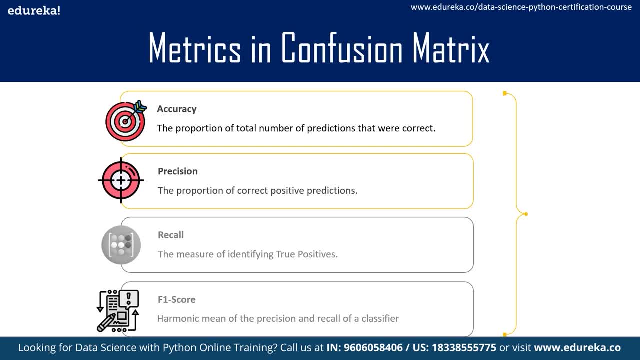 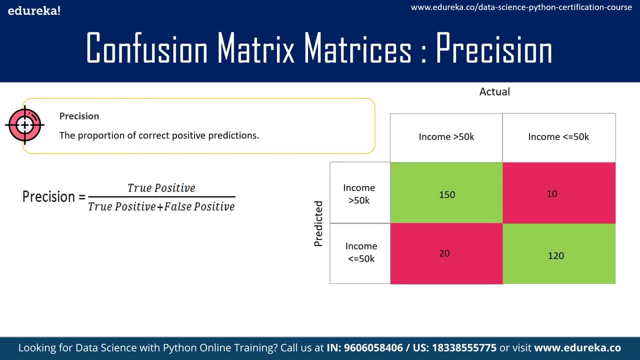 study precision. Now, precision is the proportion of correct positive predictions. What does this mean? Let us understand this Now. the formula for precision is true positive divided by true positive plus false positive. Let's fill in this formula and we get precision as 93 percent. 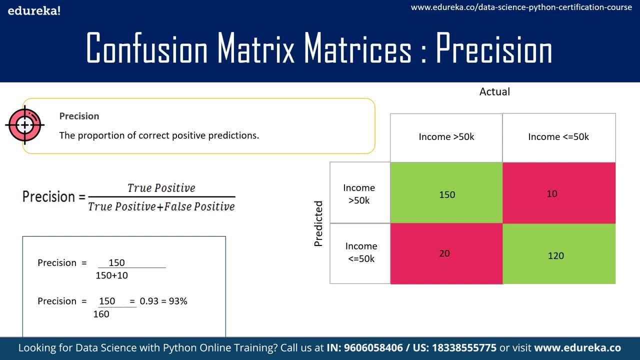 All right. so now again, the precision will tell us the correct or the positive predictions made by the algorithm. So how precise is my algorithm? So my algorithm is 93 percent precise in predicting the correct cases, but also this is seven percent incorrect because it is classifying a few cases. 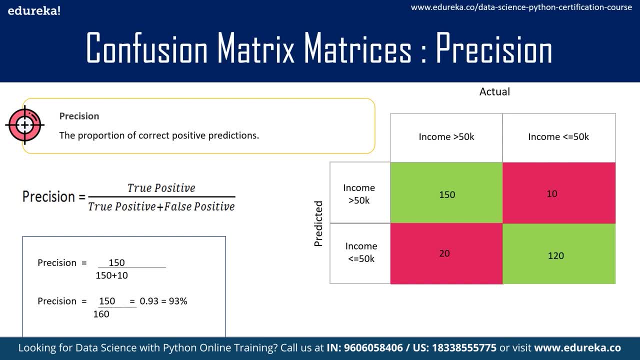 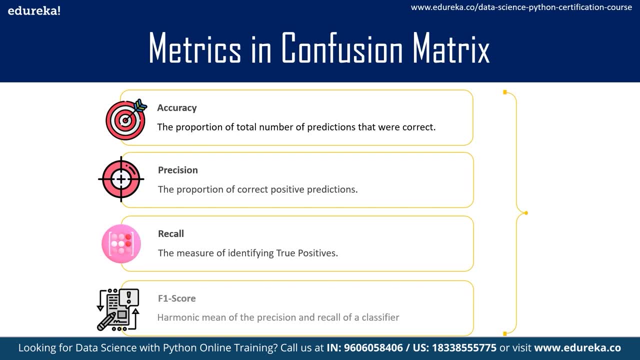 incorrectly right. So how do we map those incorrect cases? And for that we have got different matrices, that is recall, and here this is a measure of identifying the true positives. So what does this mean? Let us understand this with the help of a formula. 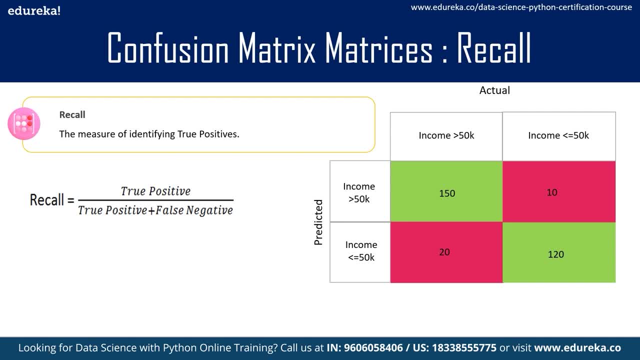 So recall formula is: true positive divided by true positive plus false negative. Let us fill in the values of this and we get, after filling the values, 88 percent recall. So what is this recall actually? This is also telling me the incorrect predictions It is taking into account. 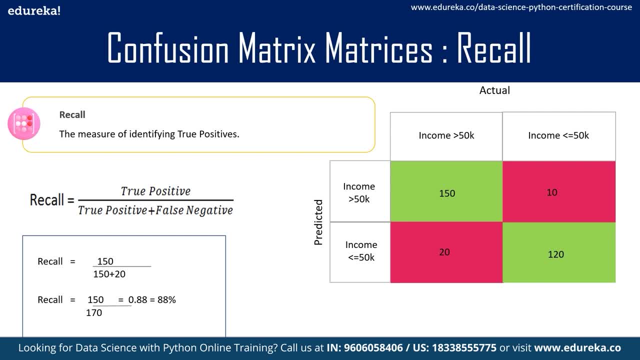 the misclassified cases, The true positive cases which will be misclassified. So it is telling me that a classifier is not that accurate because it is giving me few errors also. So recall is a measure of identifying the true positives. How many true positives? but also the cases of the true 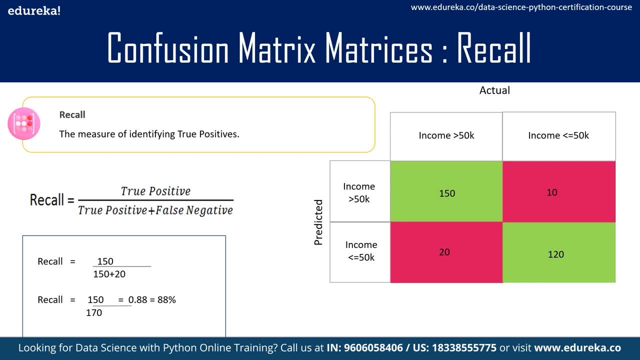 positives which were misclassified right And this is very important in healthcare sector, wherein we have seen that the patient had heart disease but the algorithm or the doctor wrongly classified. So this is telling me that the true positives which were misclassified it as not having heart disease. So that was a false, negative error and we don't want that. 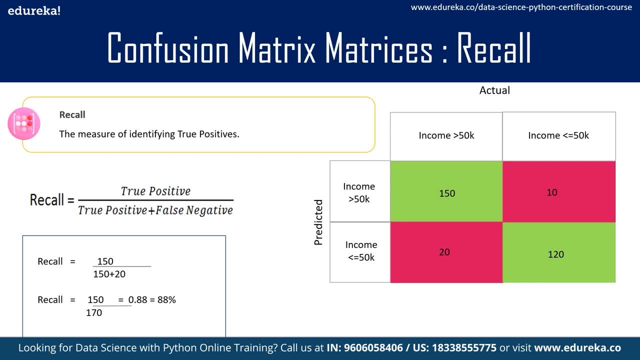 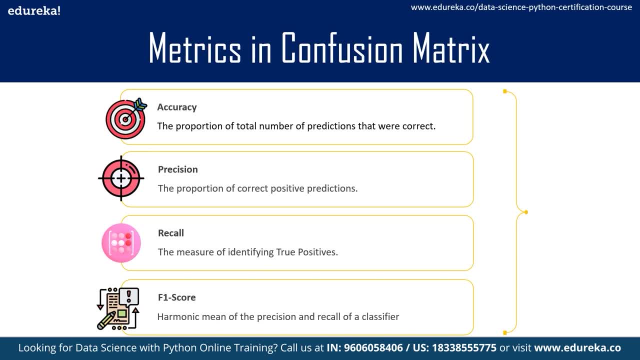 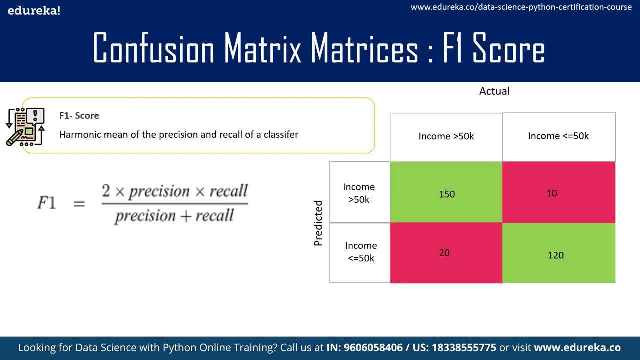 F2 load factor is another combination of precision and recall as it combines them in harmonic mean. So harmonic mean of precision and recall of a classifier is F1 score and we calculated with a formula, as F1 equals to 2 into precision, into recall, divided by precision plus recall. 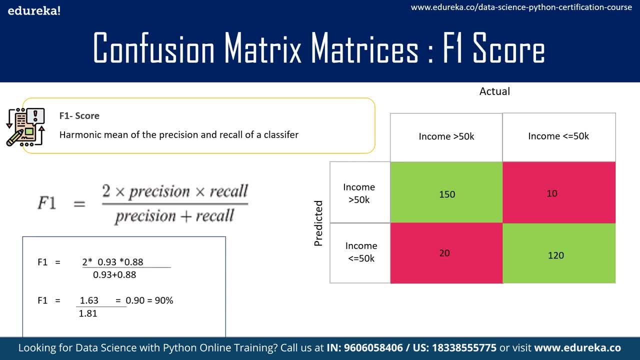 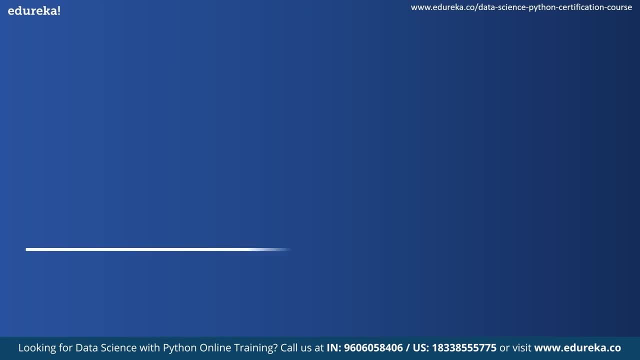 And here we see it is coming to be 90%. Okay, so this is nothing but, again, a harmonic mean of precision and recall. Now moving on forward to confusion: matrix for multi class classification: classification: All right, So this was a problem of a simple binary classification. So confusion. 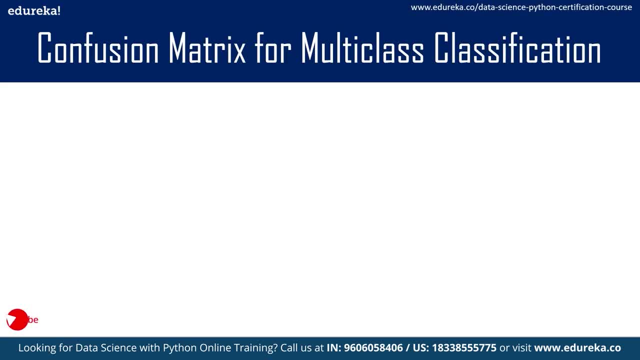 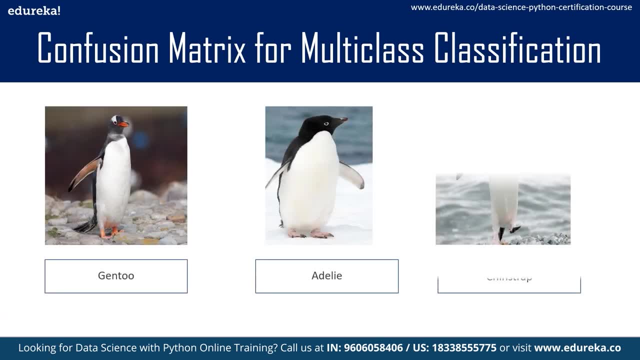 matrix was easy to interpret. But now what happens is that we've got some multi-class classification, like classifying the penguin species into Gento, Adli and Chinstrap. So now this is like three species and we have to find out true, positive and false, negative and various. 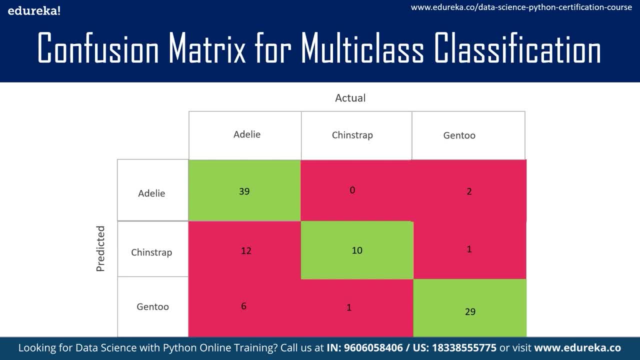 cases by the algorithm. How do we find that? So this is the confusion: matrix of a multi-class classification data set. So this was a penguin's data set. And again we can see the actual values above and in the columns we would have the predicted values. So now we see a confusion. 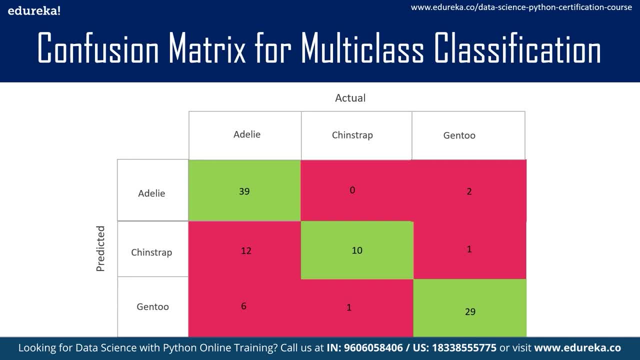 matrix for a multi-class classification And in the columns we have the actual values and in the rows again we've got the predicted values. So as you can see that the Adli when the actual and the predicted values of Adli penguin matches, that is 39. That means the algorithm correctly. 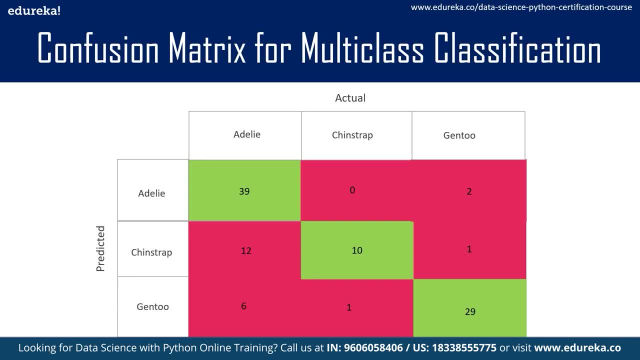 classifies 39 cases of Adli correctly. The Chinstrap and Chinstrap predicted are 10.. That means 10 Chinstrap penguin species have been correctly grouped into Chinstrap And we see Gento in the predicted. that is 29.. That means these are the correctly predicted Gento species. 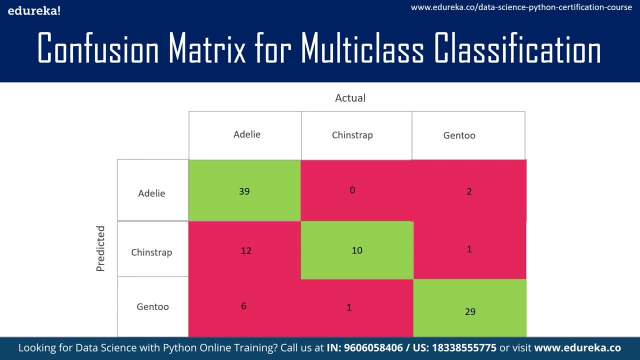 correctly classified And we can also see that the diagonal here is the Gento species. So we can see that the diagonal here is the Gento species. So we can the correct predictions made by the algorithm and the rest of the predictions are errors, or 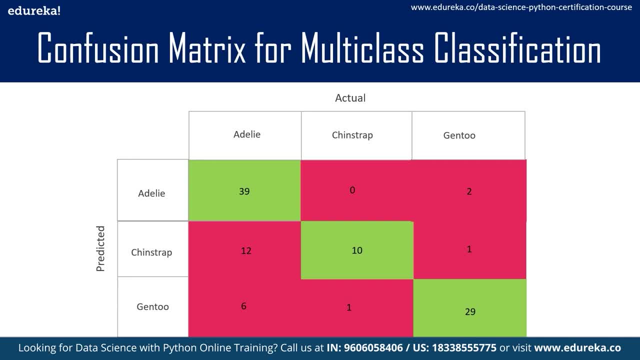 misclassified cases Now. but the question is: how would you calculate the false positive and false negative from this? So now let us understand how we will calculate various matrices and also true positive, true negative, false positive and false negative from this matrix. So now again. 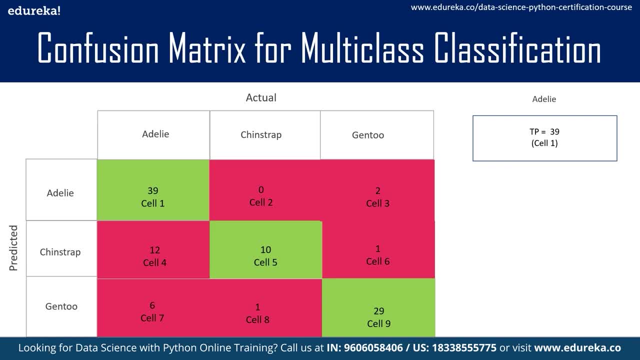 we would see for Adli, just for instance, what we have here is that true positive is 39, which is referred to as cell 1.. So for convenience sake, we have just divided these cells and given them names And cell 1, and that is 39. This is true positive for the. 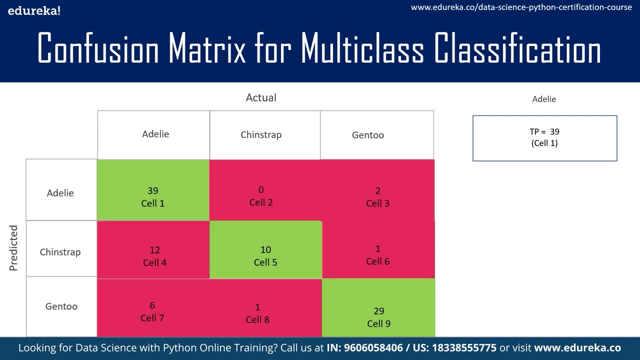 Adli class. We are just calculating the matrices for the Adli class of penguins right, And similarly this could be done for Chinstrap and Gento too. So, moving on forward with Adli, we've got false negative. How will we calculate false negative? So we are just going to calculate the false negative. 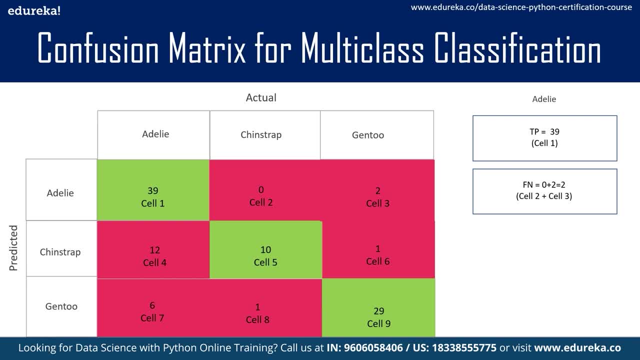 is that cell 2 plus cell 3,. that is a false negative for Adli. That means all the classes except Adli, right. Moving on forward to false positive, which will be cell 4 plus cell 7, that is 12 plus 6,, that is 18, right, These are the false positive. That means the PCU is not. 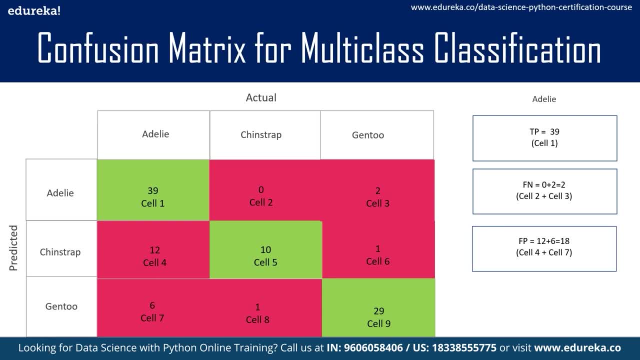 Adli, but they've been classified as different species, that is, Chinstrap and Gento right. So now coming to true negative, that means the correctly classified cases. that means the penguin species which were not Adli, and they were correctly classified. So 41 cases were. 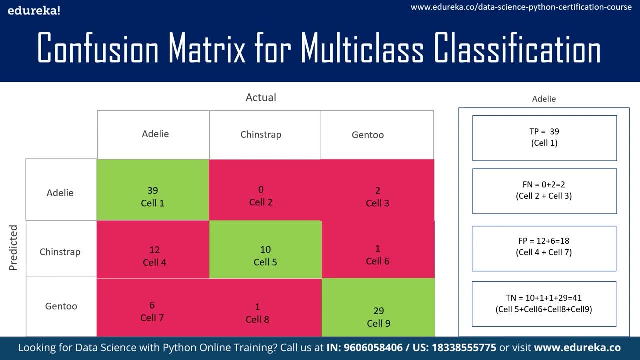 being correctly classified. They were Chinstrap and Gento and it was not Adli. So these were the true negative. So true negative and true positive are the correct prediction made by our algorithm. Now moving on forward to calculating a few matrices here. So now let us calculate the. 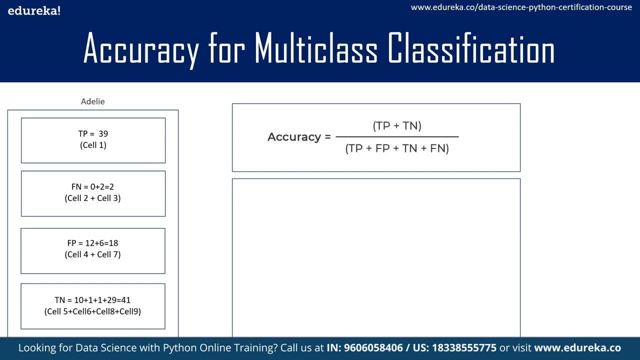 accuracy for the confusion matrix. So now we have accuracy as true positive plus true negative divided by the total number of cases. So we have true negative and true positive. So we have true negative and true positive. So we have true negative and true positive. So the accuracy comes out to: 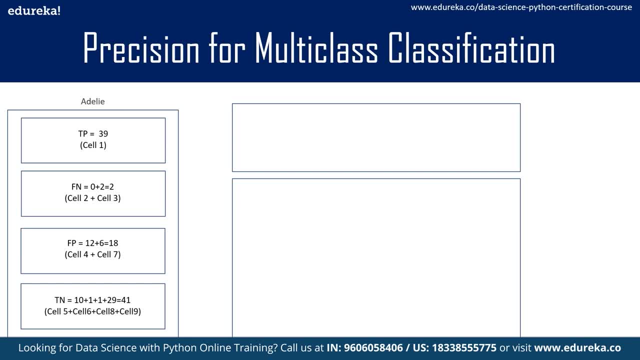 be 80% after filling these values. Now moving on forward to precision, and precision is true positive divided by true positive plus false positive. So precision comes out to be 68%. And now coming to recall, which is true positive divided by true positive plus false negative, And the recall. 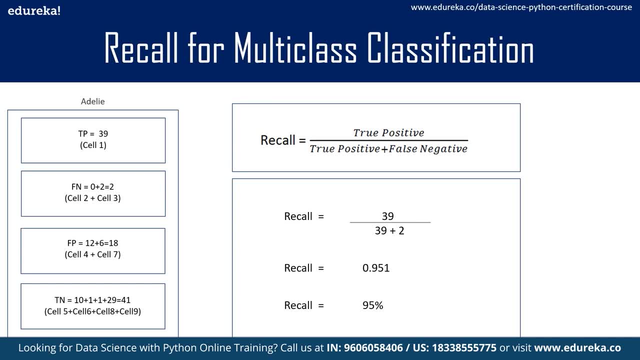 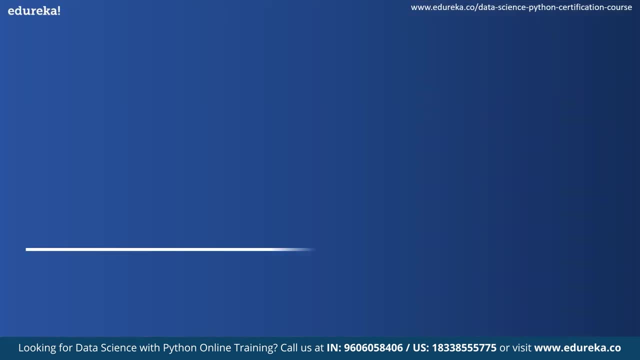 after filling the values from confusion matrix, we get recall as 95%. All right, so this was all about the multi-class classification and how do we actually find out various matrices from the confusion matrix? Now moving on forward to key points in confusion matrix. So this is the summary and the 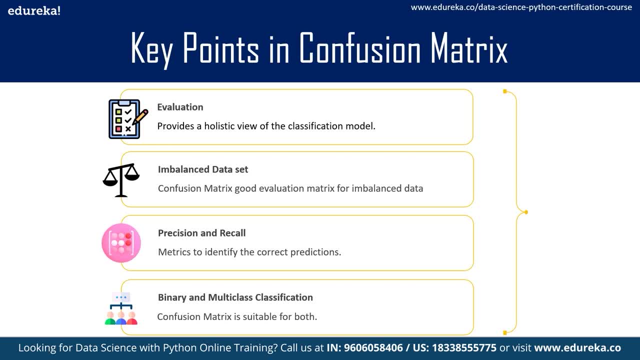 consolidation of everything that we have learned so far. So the essence of confusion matrix is evaluation: that it provides a holistic view about the classification model and how is it performing and what all are the errors that the model is making. So if our imbalance data set. 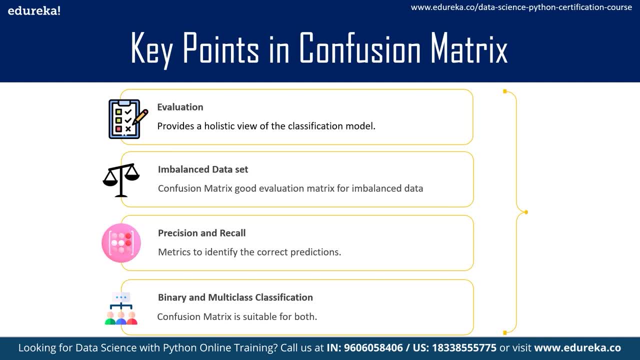 also confusion. matrix gives a good evaluation matrix, unlike accuracy, which is suitable for balanced data set And in real life we mostly encounter the imbalanced data set. Now moving on forward to precision and recall the matrices to identify the correct predictions and confusion.